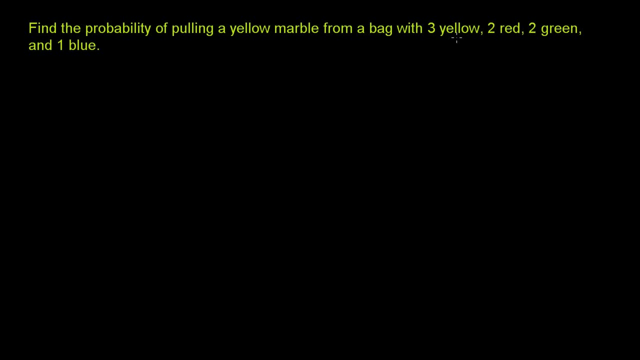 Find the probability of pulling a yellow marble from a bag with three yellow, two red, two green and one blue, I'm assuming marble. So they say the probability. I'll just say P for probability: the probability of picking a yellow marble. 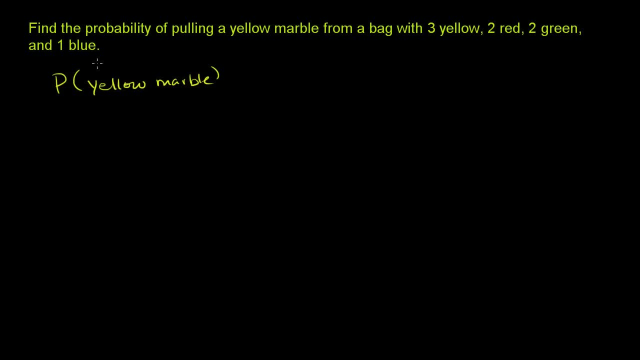 And so this is sometimes the event in question right over here is picking the yellow marble. I'll even write down the word picking, And when you say probability, it's really just a way of measuring the likelihood that something is going to happen. 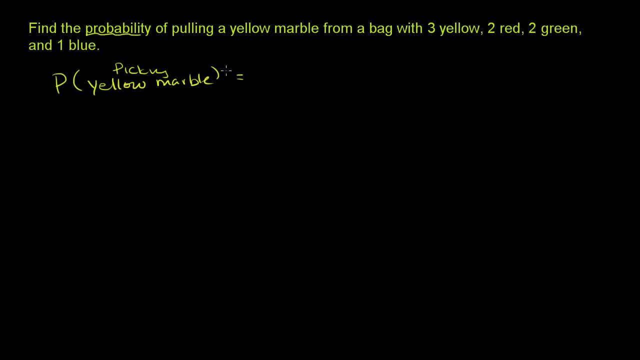 And the way we're going to think about it is how many of the outcomes from this trial, from this picking a marble out of a bag, how many meet our constraints, satisfy this event and how many possible outcomes are there. So let me write the possible outcomes right over here. 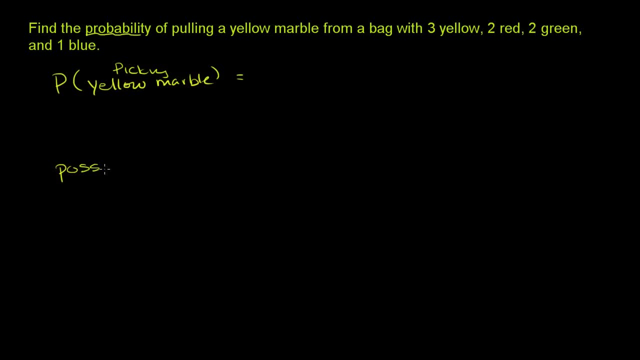 So possible outcomes, And you'll see, it's actually a very straightforward idea, but I'll just make sure that we understand all the words that people might say. So the set of all the possible outcomes, Well, there's three yellow marbles. 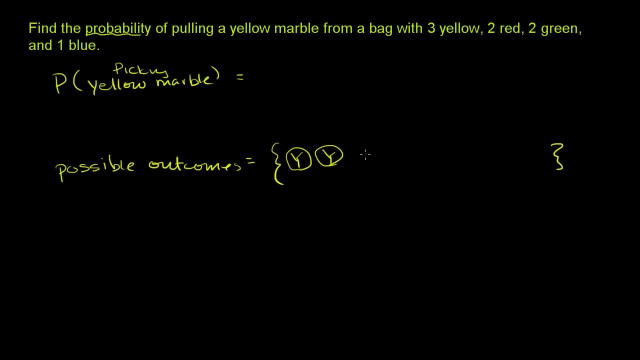 So I can pick that yellow marble, that yellow marble or that yellow marble. These are clearly all yellow. There's two red marbles in the bag, so I could pick that red marble or that red marble. There's two green marbles in the bag, so I could pick that green marble or that green marble. 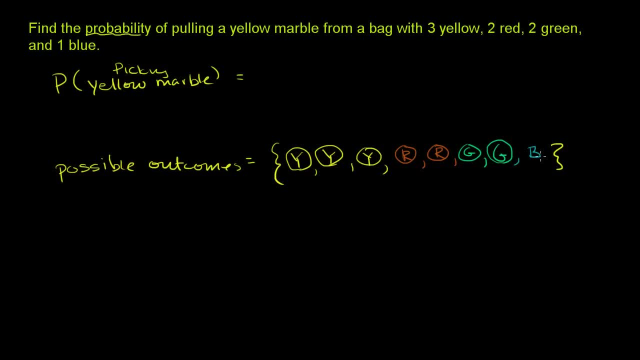 And then there's one blue marble in the bag. So this is all the possible outcomes. outcomes, and sometimes this is referred to as the sample space sample, the set of all the possible outcomes- fancy word for just a simple idea that the sample space if when I pick something out of the bag and that picking out of the bag is 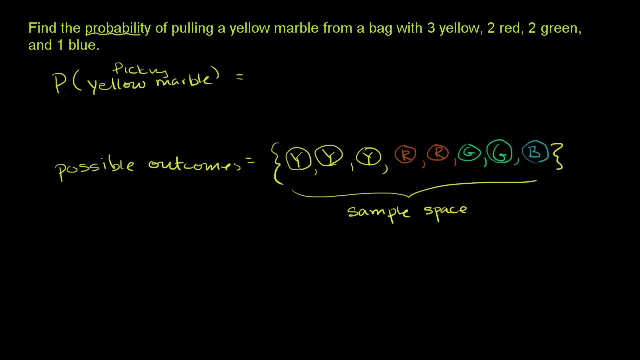 called a trial. there's eight possible things I can do. so I think about the probability of picking a yellow marble I want to think about: well, what are all of the possibilities? well, there's eight possibilities, eight possibilities for my trial. so the number of outcomes, number of possible outcomes, you could view it. 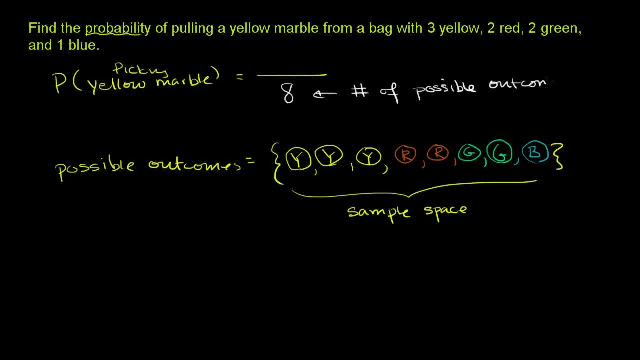 as the size of the sample space, number of possible outcomes, and it's as simple as saying: well, look, I have 8 marbles. and then you say, well, how many of those marbles meet my constraint that satisfy this event here? well, there's three marbles that satisfy my event. there's three outcomes that that will allow this. 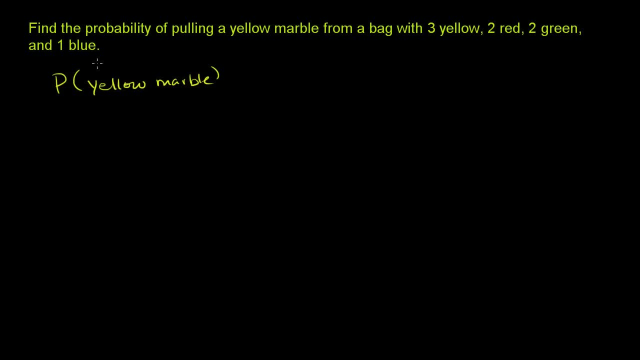 And so this is sometimes the event in question right over here is picking the yellow marble. I'll even write down the word picking, And when you say probability, it's really just a way of measuring the likelihood that something is going to happen. 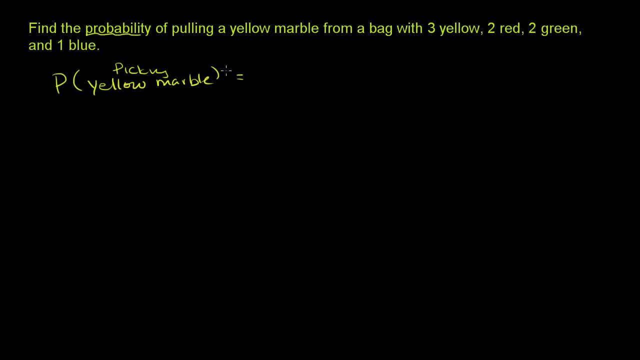 And the way we're going to think about it is how many of the outcomes from this trial, from this picking a marble out of a bag, how many meet our constraints, satisfy this event and how many possible outcomes are there. So let me write the possible outcomes right over here. 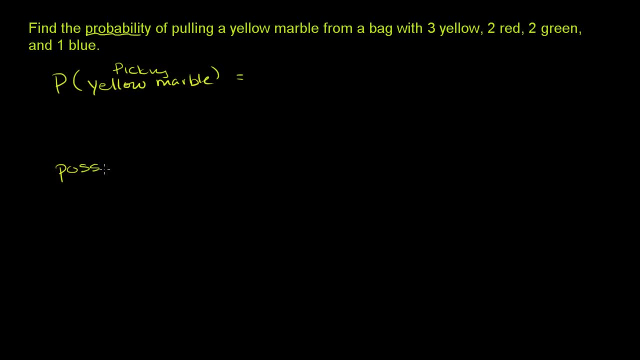 So possible outcomes, And you'll see, it's actually a very straightforward idea, but I'll just make sure that we understand all the words that people might say. So the set of all the possible outcomes. Well, there are three yellow marbles, so I could pick that yellow marble, that yellow marble or that yellow marble. 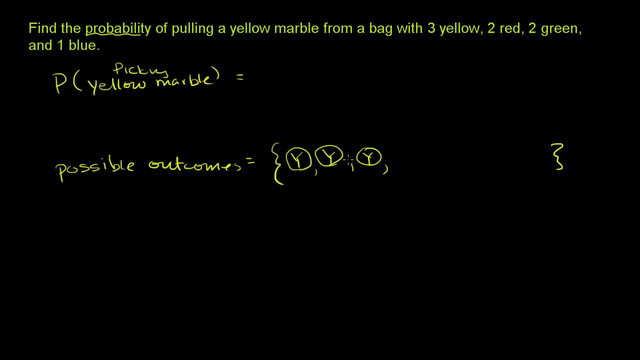 These are clearly all yellow. There's two red marbles in the bag, so I could pick that red marble or that red marble. There's two green marbles in the bag, so I could pick that green marble or that green marble. And then there's one blue marble in the bag. 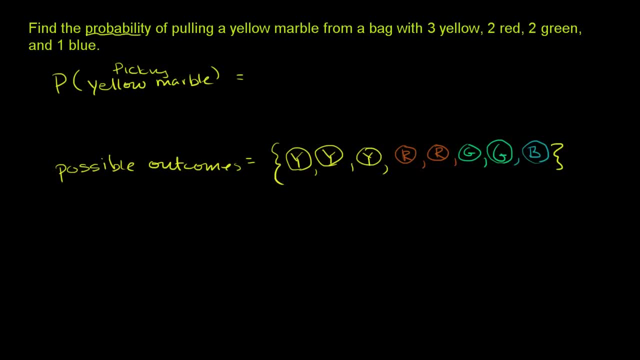 So this is all the possible outcomes. outcomes, and sometimes this is referred to as the sample space. sample, the set of all the possible outcomes. fancy word for just a simple idea that the sample space if when I pick something out of the bag and that picking out of the bag is- 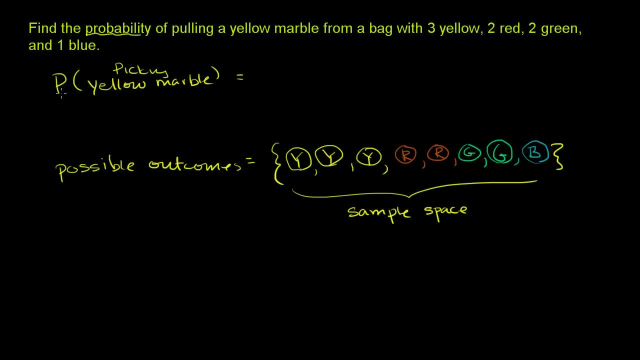 called a trial. there's eight possible things I can do. so I think about the probability of picking a yellow marble I want to think about: well, what are all of the possibilities? well, there's eight possibilities, eight possibilities for my trial. so the number of outcomes, number of possible outcomes, you could view it. 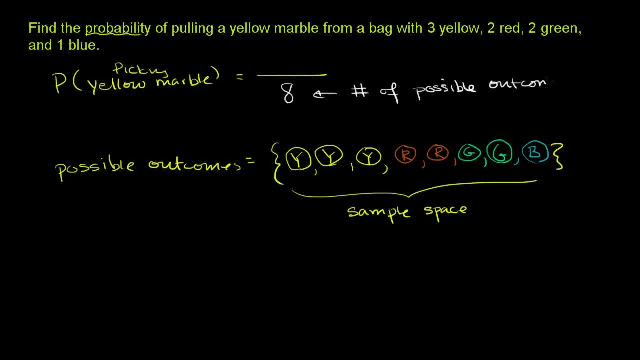 as the size of the sample space, number of possible outcomes, and it's as simple as saying: well, look, I have eight marbles. and then you say, well, how many of those marbles meet my constraint, that satisfy this event here? well, there's three marbles that satisfy my event. there's three outcomes that that will allow this.